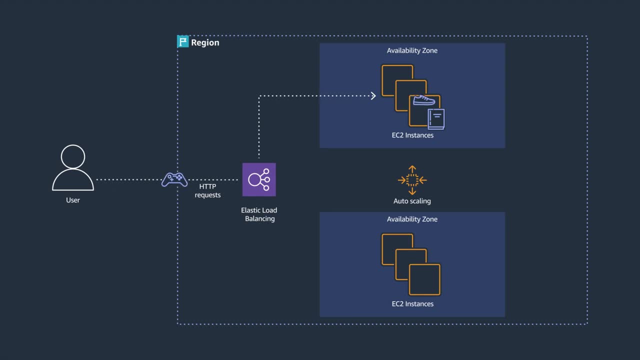 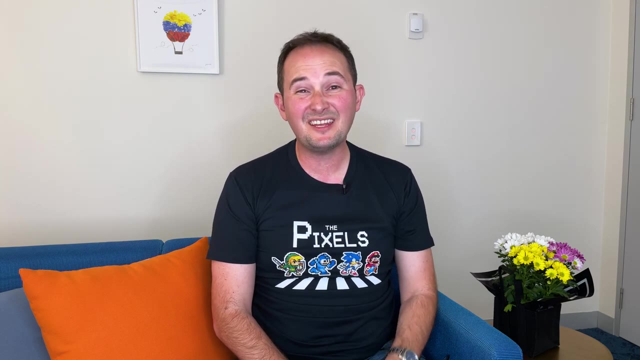 the web application remembers what is the easy-to-instance that is serving a particular customer at a time. The advantage of this approach is simplicity: You can set up sticky sessions just going into the AWS console and clicking a checkbox. What are the disadvantages of this approach? 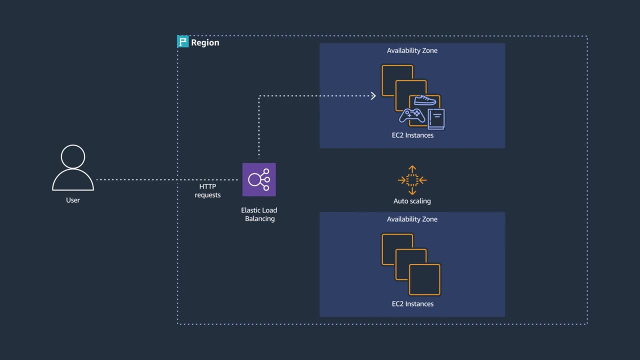 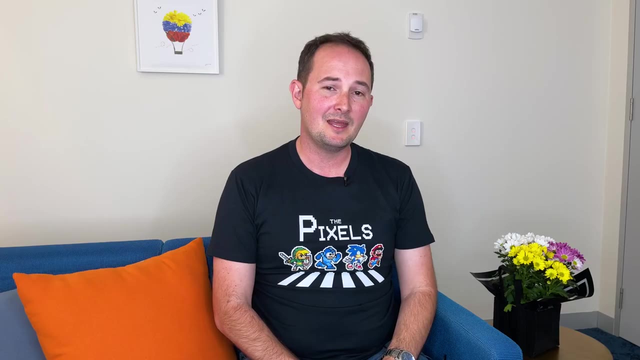 It's always a good practice to anticipate failure. What's happening if a server is going down? A lot of people forget that if you deploy a new version of the product, all the sessions living on that server are going to be lost. And let's think a little bit more If you want to deploy a new version of your product. 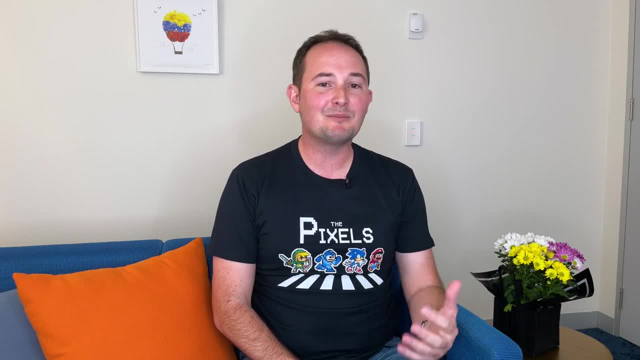 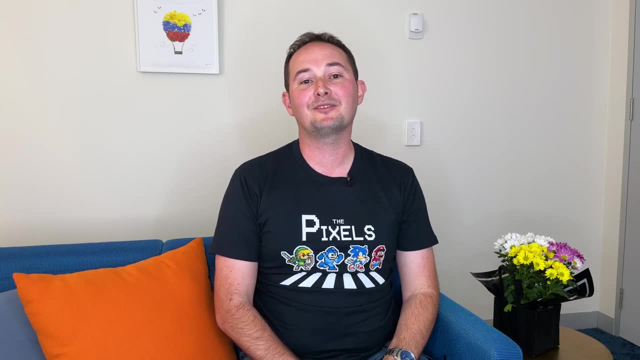 how are you going to do it? Blue-green deployments- canary deployments. Remember, if the server is going down, your sessions are going to be lost, impacting some of your customers. If you saw that, having your session data in your easy-to-instances is super simple, 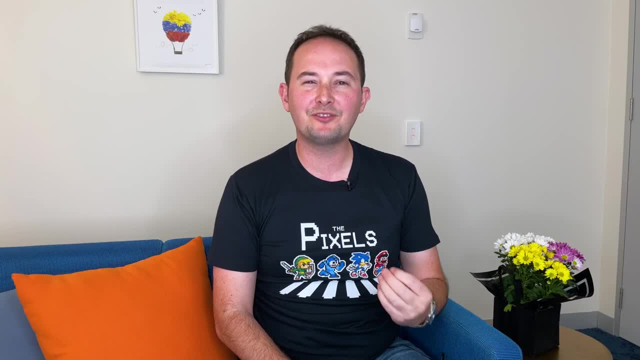 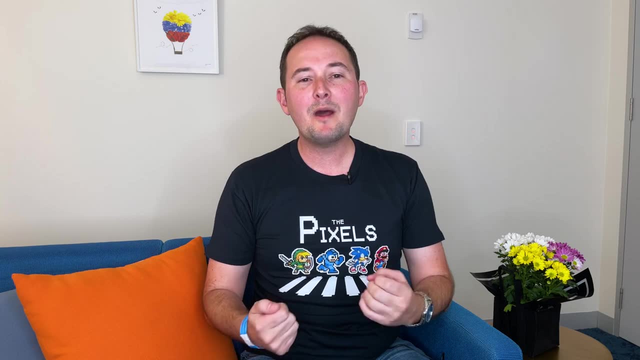 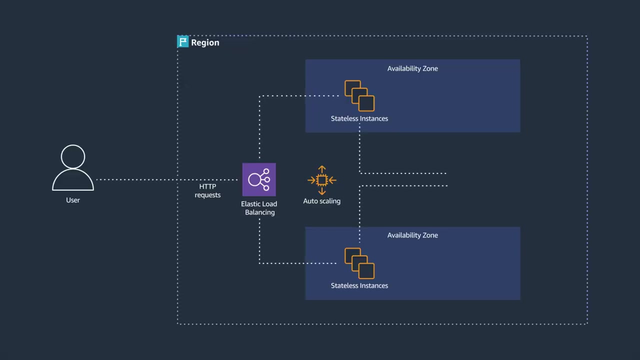 but it has some disadvantages. Is there any way to make your services stainless so you decouple your session data from your EC2 instances? What about having a distributed cache out of your EC2 instances, keeping the session data As you can see in this architecture? 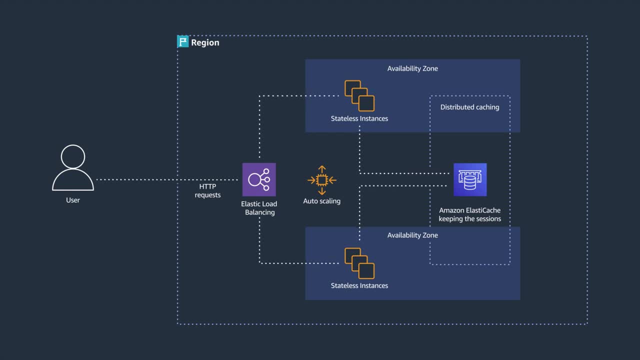 you can leverage an in-memory key value store, such as Redis or MainCache. This approach adds some complexity to the solution, but it's abstracting the sessions from the web service themselves. Key value data stores are extremely fast and provide sub-millisecond latency. 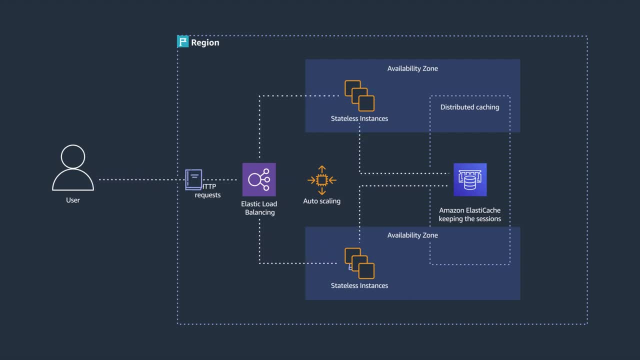 Whenever a server wants to modify the session, the service will not keep the change in its local memory. It will make the change in Elastic Cache That makes your services stainless, which is considered a best practice, Even better if a server is going down. 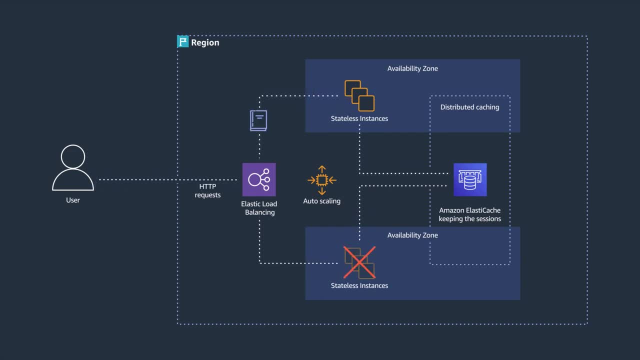 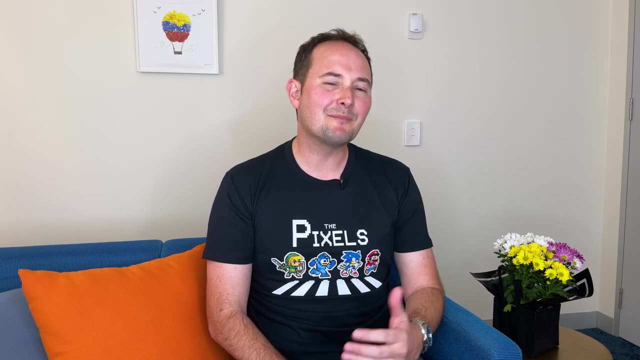 or you need to perform a new release of your code. your customers are not going to be impacted. There are some particular cases where you want to use sticky sessions, For example, if you have a legacy application that is relying on your sessions being in the servers. 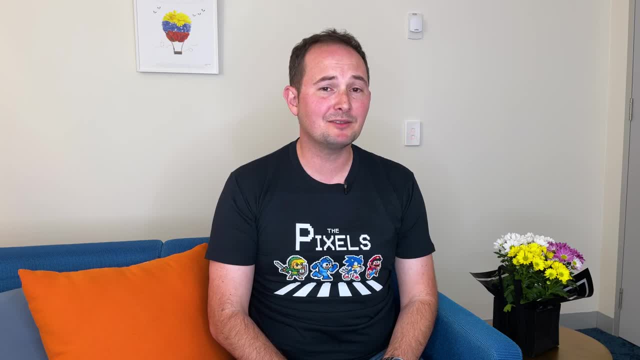 However, in most of the cases, I prefer to have my web sessions in a distributed cache. In that way, your application becomes more reliable and your deployments become simpler. Check the links below for more details. Thank you for watching Back to Basics.